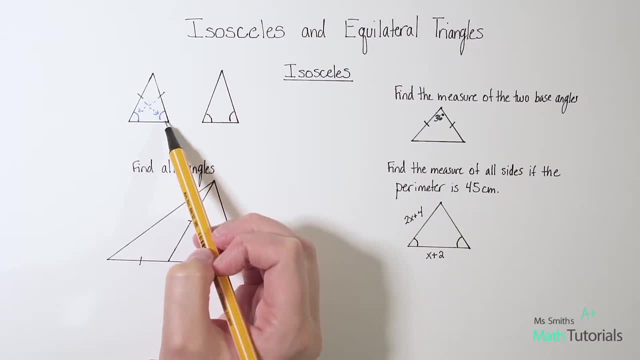 equals this angle, right? That's not what we're saying at all. We're saying that in an isosceles triangle, these two sides would be equal to each other. These two angles will be equal to each other. Okay, So sometimes all they'll give you is a tick mark. Okay, Sometimes all they'll give you. 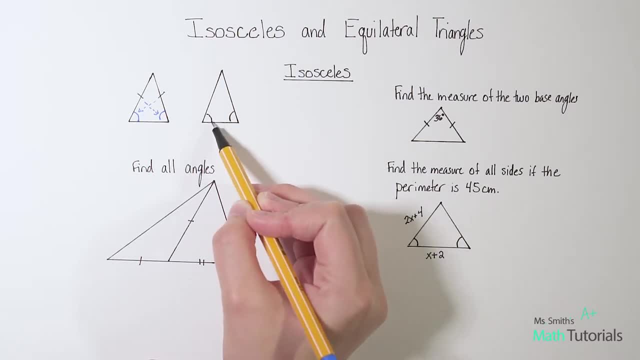 is this little, these little base angles. These are like tick marks, but for angles. Okay. So when you see a matching set like that, that means these two are congruent, They are equal to each other And, if I can say, these two. 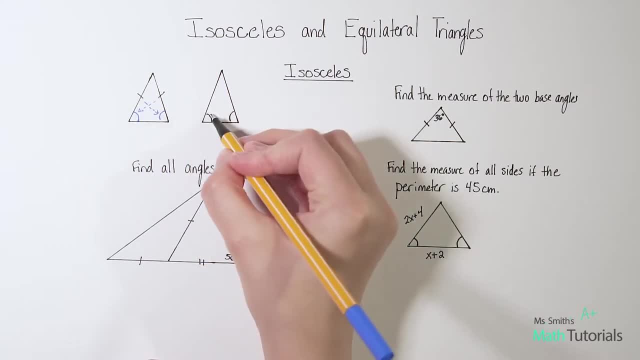 are equal to each other, then I can do the reverse of what I just did. I can say: well, I also know that the matching sides are congruent to each other. Okay, So sometimes they'll show you both, They'll give you both the tick mark, as well as this: 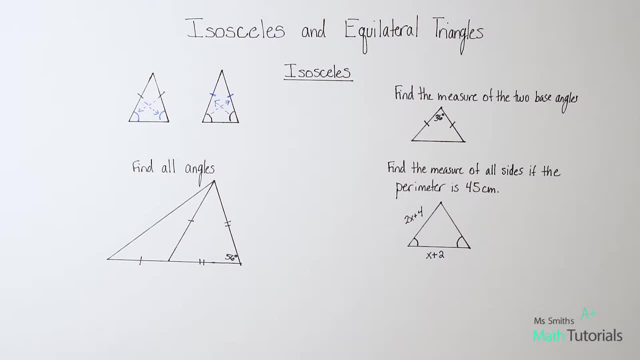 Sometimes they will give you none of the above and they'll just tell you it's an isosceles triangle. But usually, usually, they'll give you either this or this and you've just got to understand that. what assumptions you can draw from that? So let's look at some problems related to 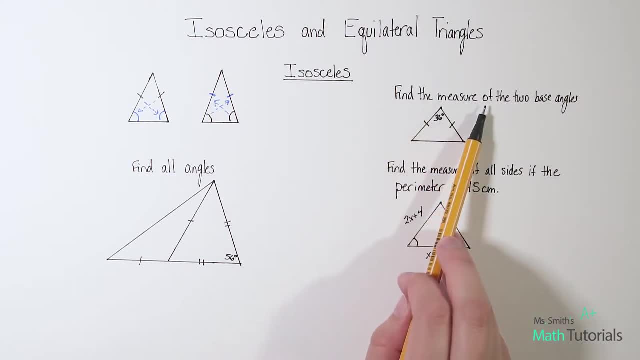 isosceles triangles. This first one says: find the measure of the two base angles. So let's look at what they've given me. I've got this triangle. I see a tick mark here and here. Now they're telling me that the top angle is 36 degrees. Now that top angle? okay, it's not one of. 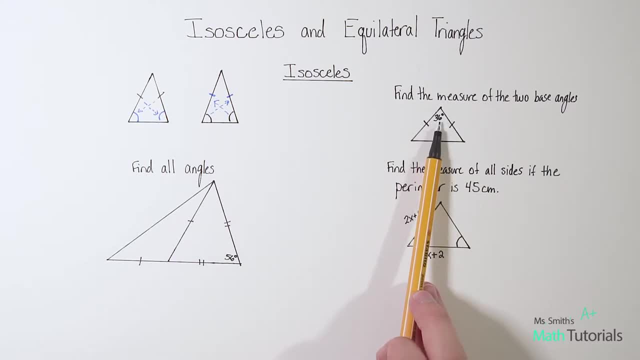 the base angles. It's the kind of odd ball out, if you will, That is called the vertex angle of the triangle. So just be aware that's a good term to know. So if this is 36 and these two are congruent, then I can say that the top angle is 36 degrees. So if this is 36 and these two are, 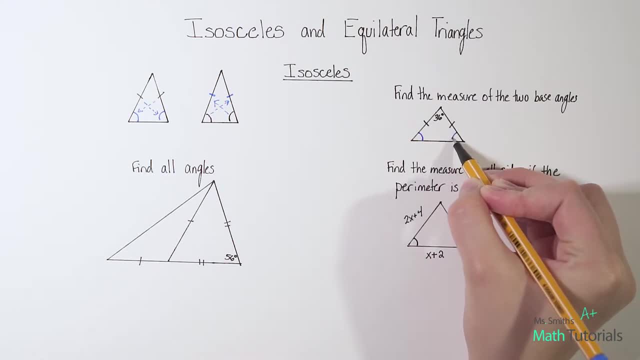 congruent, then I can say that this angle is congruent to this angle. If I know the top angle is 36, I have to think back to what I know about the angles of a triangle, And I know the angles of any triangle add up to give me 180 degrees. So if I know one of the angles is 36, let me see. 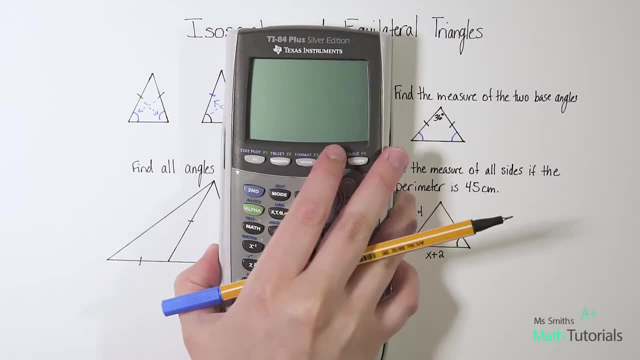 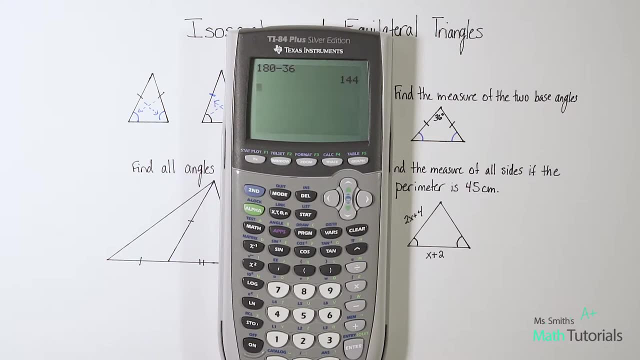 what the difference would be. So let's do 180.. 180 minus the one angle, I know 36.. All right, I get 144.. Now I know that 144 has to be split evenly between here and here, because these two are equal, They're congruent to each other. So it has. 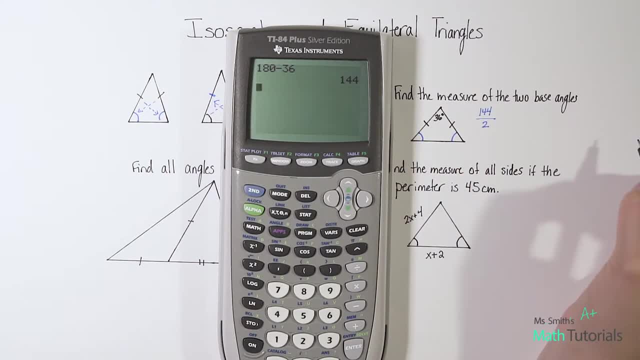 to be split right down the middle. Okay, and that means divided by two. So let's do 144. divided by two, I get 74. So that tells me that this angle is 72 degrees, and this angle is 72 degrees And I can mark it on. 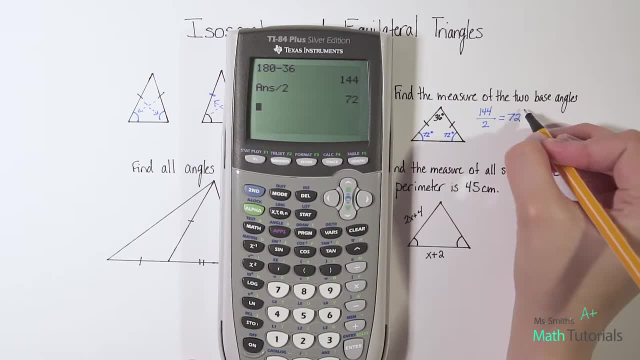 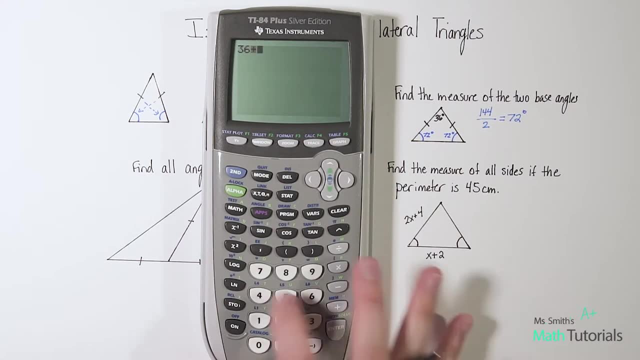 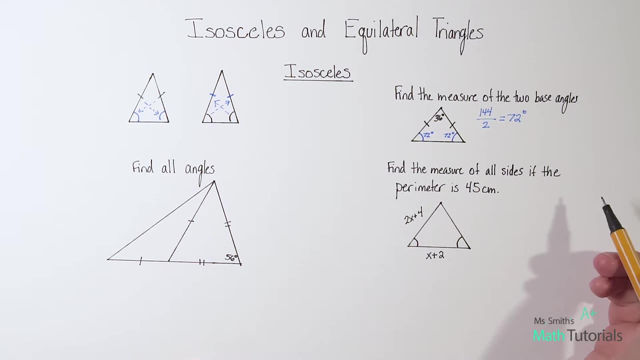 there. if I want Right And we know, our answer is 72 degrees each. And then you can always double check yourself: 36 plus 72 plus 72. And you should get 180.. Always good to double check yourself to make sure you didn't make a careless error. 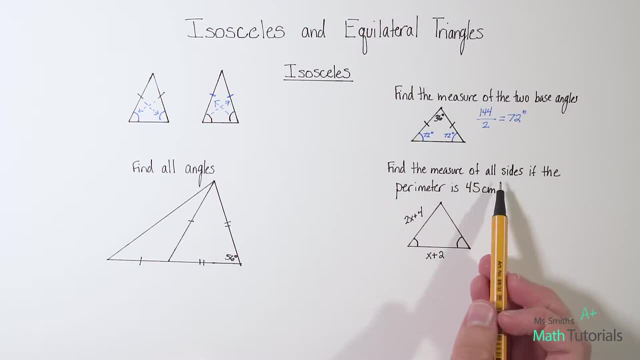 Let's look at this one down here. Find the measure of all sides if the perimeter is 45 centimeters. Now a couple things I got to recognize about this. What does perimeter mean? Remember that perimeter. I always think of it like fencing, right So in my backyard. if I wanted to know. 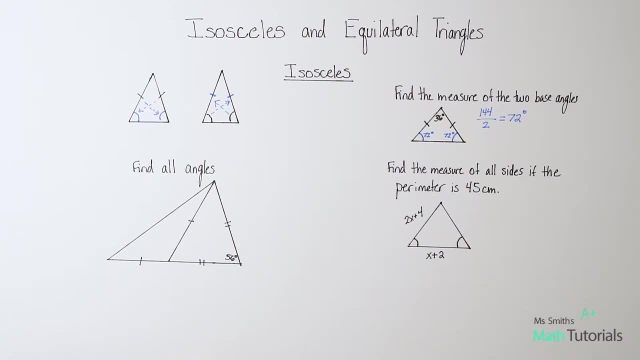 the perimeter of the fence. I'm adding up the whole length, Like if my backyard was triangle shaped, right Then I would be adding up the perimeter of the fence. So if I wanted to know the fence line, okay, I'm not adding up the center, I'm not finding, I'm not multiplying to find the 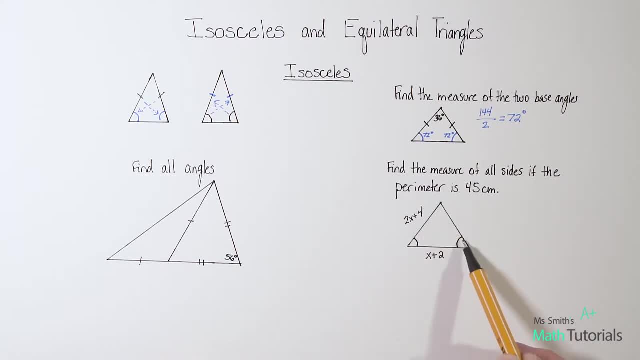 area. Okay, I'm just adding the outer lining. Okay, so they're telling me that the perimeter of this whole thing is 45 centimeters, All right. and they've told me this side is 2x plus 4.. This side- they have not told me what it was directly- And this base is x plus 2.. Now the fact: 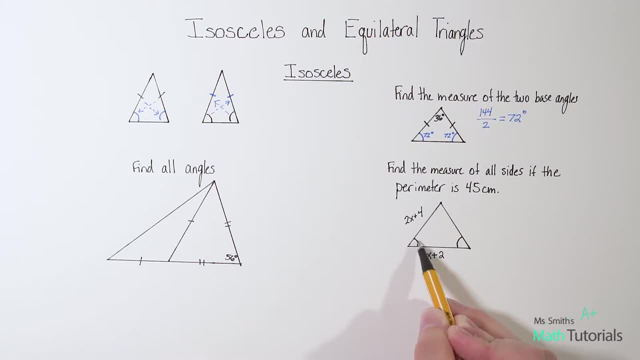 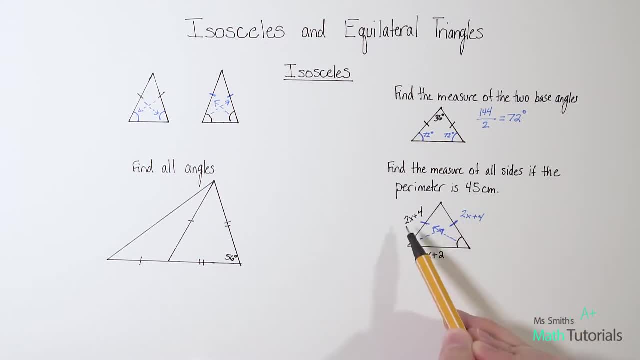 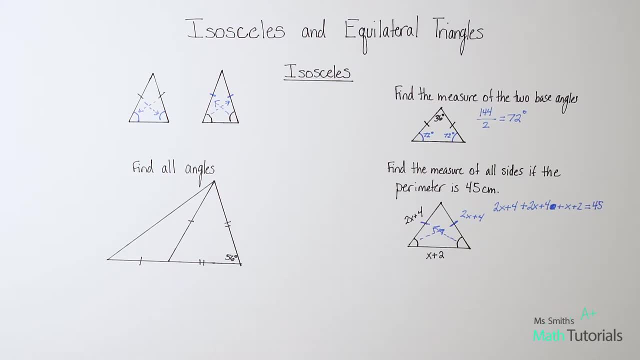 equals 180, because they get so caught up in thinking triangles mean 180. Well, the interior angles add up to 180, not the sides. The sides could add up to almost anything, right, But the angles add up to 80.. So, please, please, if you were tempted to say equals 180 here, that's something. 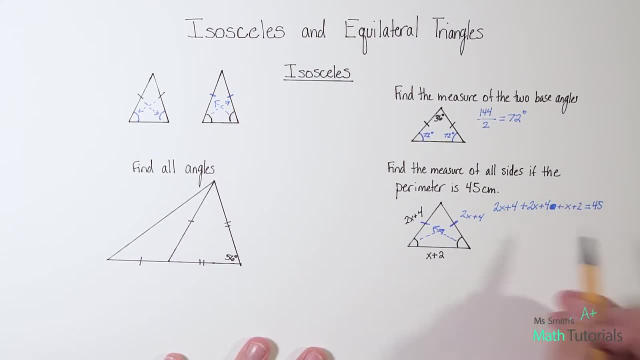 you really need to be careful of. okay, It equals the perimeter, So let's do a little combining like terms: I've got 2x plus 2x plus x, So that's going to be 5x, And then I've got 4 plus 4 plus 2.. So 8,. 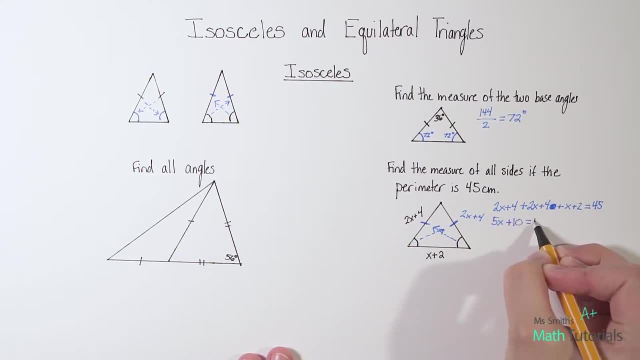 9, 10.. So 5x plus 10 equals 45. I want to subtract 10 from both sides to get x alone. 45 minus 10 is going to give me 35. I need to divide out that 5. And I get x equals 35. divided by 5 is 7.. Okay. 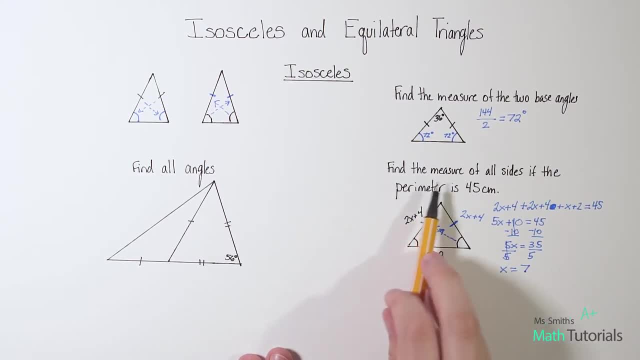 now I need to be careful here, because they didn't ask me what is x? right? They said: find the measure of all sides. So I need to be able to say what is this side, What is this side And what is this side? And they're not 7, right, I've got to plug 7 in. So I need to be able to say what is this side. 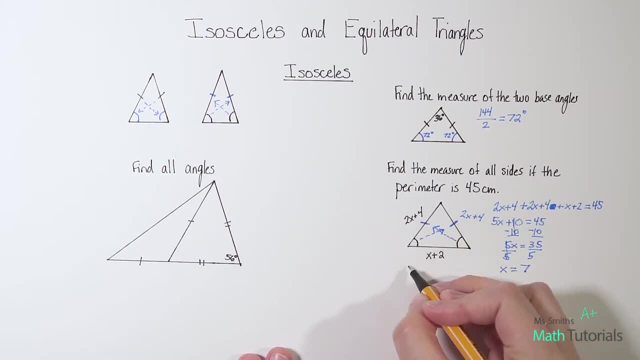 7 in for x. So for the first one let's see 2x or- sorry, it wouldn't be x- it's going to be 2 times 7 plus 4.. And 2 times 7 is 14 plus 4 is going to give me 18.. So that means this side is 18.. And 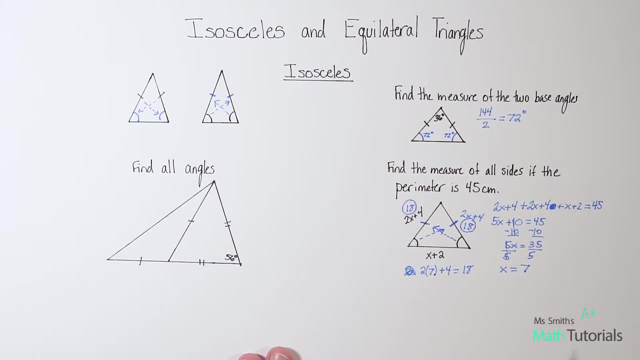 this side is 18.. They are congruent to each other. Now, for down here, I would just say 7 plus 2.. Right, And 7 plus 2 is 9.. So I know this base is 9.. For this one, it asked me to find all the. 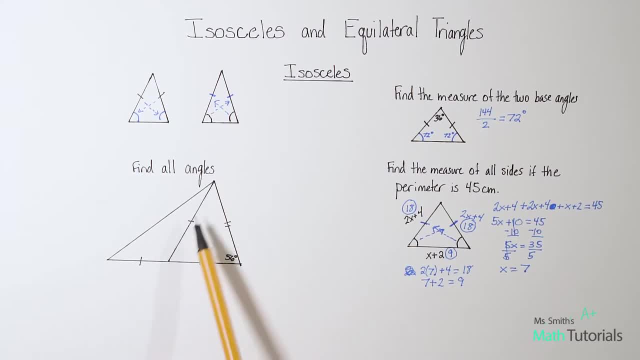 angles. So I need to be able to say what every single one of these angles are, And they've only given me one angle. I only know that this one is 56, right, But these tick marks are going to guide me with what I need to do. 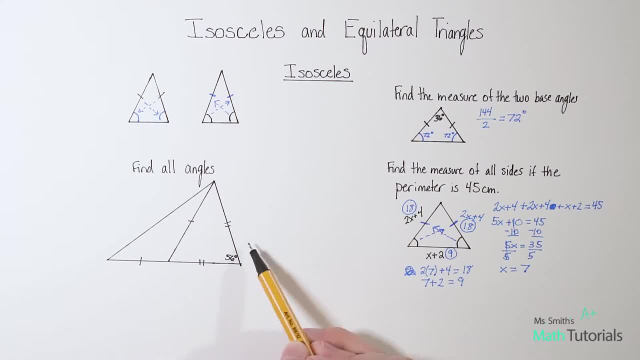 So if I know, let's just start over here with this section- that I do know. I'm not even going to look at this triangle yet because I don't have enough information. I don't know anything about that side yet, But I know. 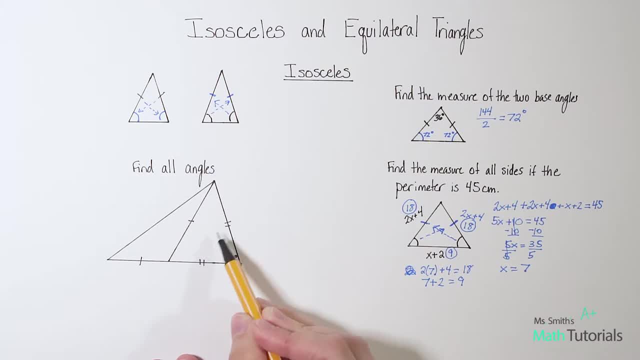 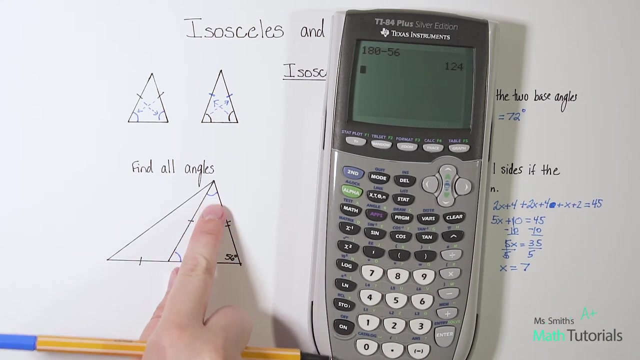 that this corner is 56. So when I see these tick marks I've got to think back to this. okay, That if these tick marks are congruent, then I know that this angle is congruent to this angle. So if I know the top angle- or, excuse me, it's not the top, it's on the side- but that vertex angle is 56, then I need to figure out what is 180 minus 56. I get 124, which has to be split evenly between those two angles. 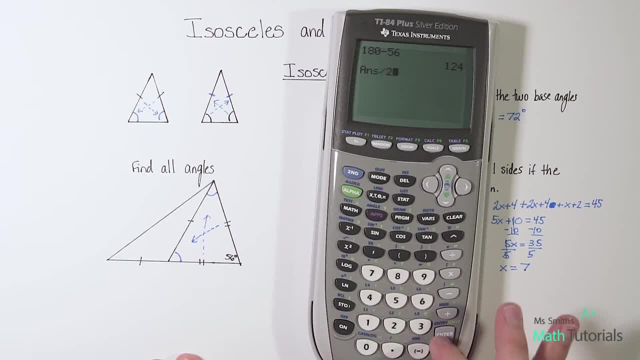 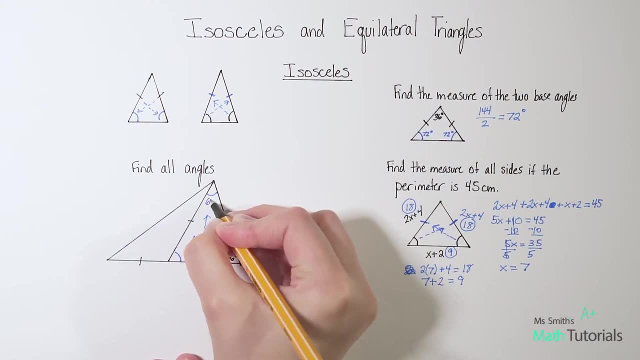 Okay, so 124 divided by 2. That's going to give me 62.. So that tells me that this angle is 62 degrees and this angle is 62 degrees. Now, one thing that I want to point out is that these have a double tick mark. okay, So that's different from the single tick mark, And sometimes you'll even see a triple tick mark, And it's just showing that these two that match, they're congruent. 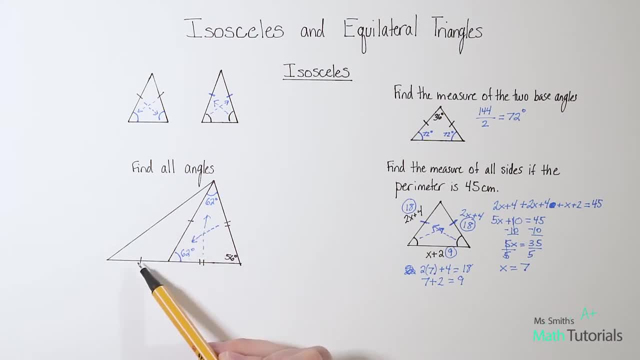 These two that match totally separate And they're also congruent to each other, okay. So just a good thing to know. Okay. so if I know this is 62, I've got to recognize that this is 180 degrees. okay. So if I know this is 62 degrees, I've got to recognize that this is 180 degrees. okay. So we have to go back to that first video, when we talked about parallel angle. 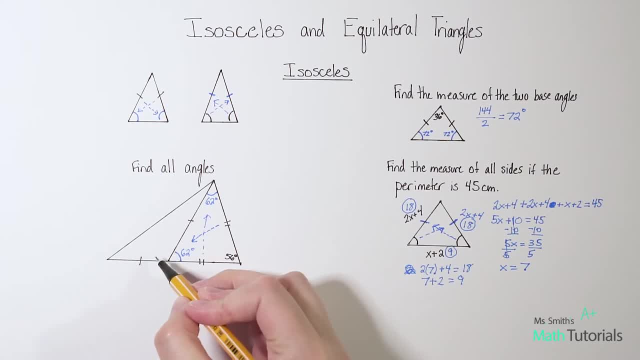 relationships. okay, That if I can do like a little rainbow here against a straight line, that whatever the angles are that make up, whatever the angle is, There is no 개� in you given this line today. I know, you know what I'm saying. I know that in fact, you know why I like this. 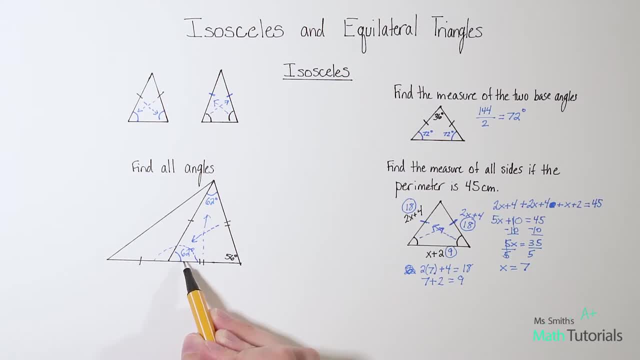 Okay, Everybody knew about this rainbow And you just say two days ago, let's go back and figure about it. Okay, the rainbow lead to 180 degrees. so if i know this is 62, i just want to know what is 180. 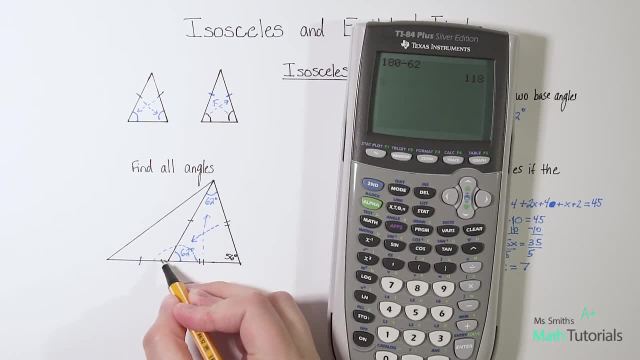 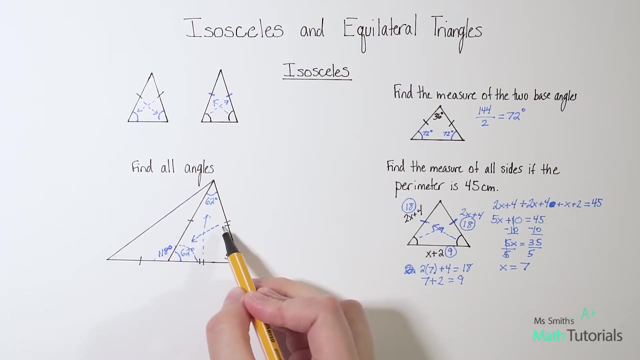 minus 62 and it will tell me the other angle, 118. so i know this angle has to be 118 degrees. all right. now, if i know this one's 118- and i see these tick marks, remember it's the same. it's just kind of like this one. i know that this angle is going to be congruent to this angle, all right. so. 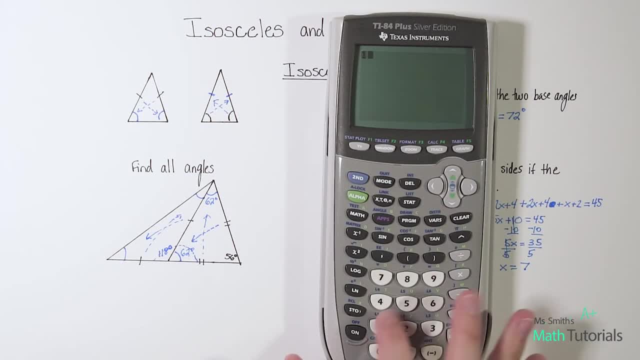 i want to take 180 again. subtract the one angle i know, because now i'm done with this triangle, really now i'm just focused on this one. so subtract the one angle i know and now take the remainder and divide it by two, because i know it's going to be a triangle and it's going to be. 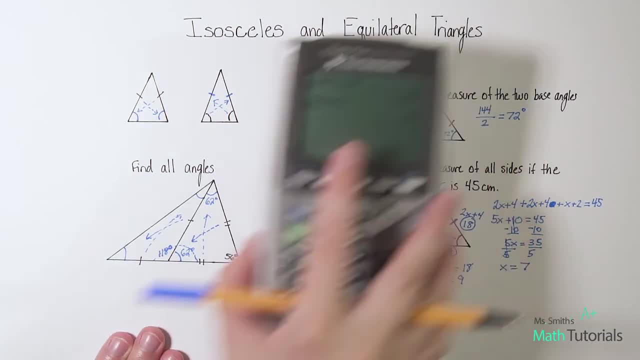 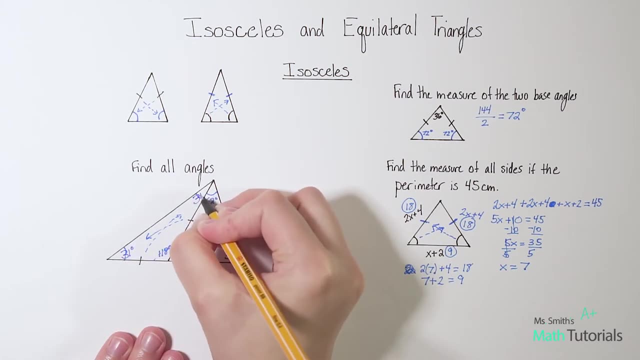 be split evenly, So 31.. So that tells me this angle is 31 degrees and this angle is 31 degrees. So I was able to figure out all the angles based off of just one corner angle, knowing it's comprised of isosceles triangles. On this page we're 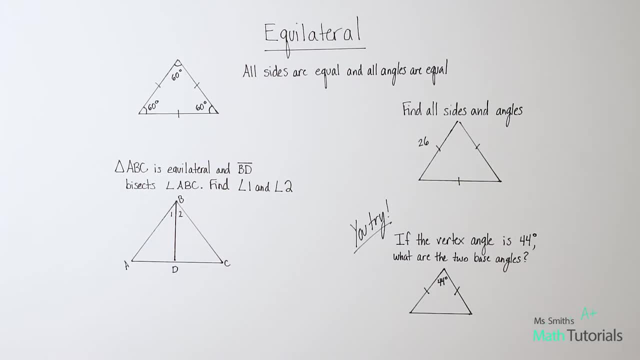 going to be talking about equilateral triangles. The thing about equilateral triangles is that all sides are equal and all angles are equal. Now let's make sure we understand the difference. When we say all sides are equal, notice how I have a tick mark on every single side. That means that whatever this side is, 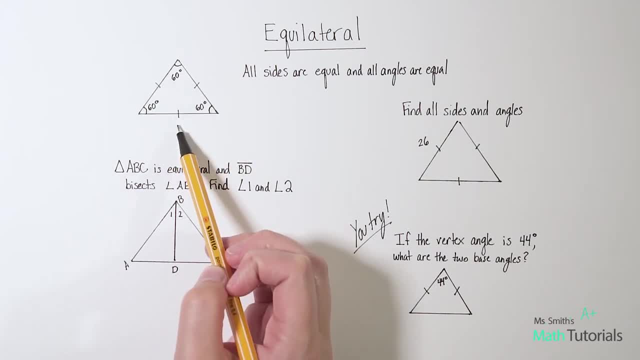 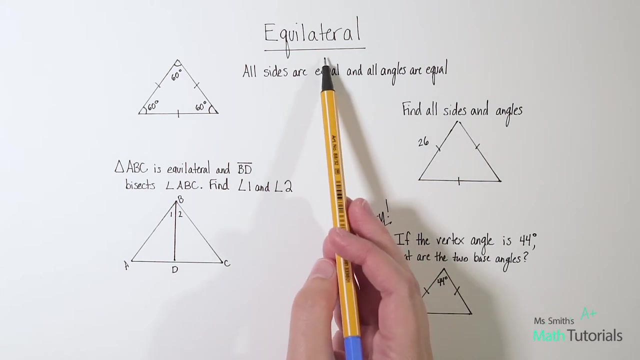 it's equal to this side and it's equal to this side. Okay, separately, all angles are equal. and for a hundred and eighty degrees to be split equally three ways, it's going to be 60 degrees every single time. So if they tell you it's an equilateral triangle, 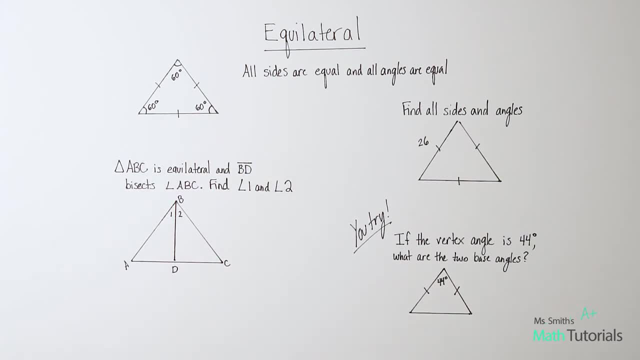 you know what the angles are. There are 60 degrees each. Okay, so just please understand that we're not saying that because these are all 60 degrees, so we're the outside. No, no, no, no, no. We don't know what the outside are. It could. 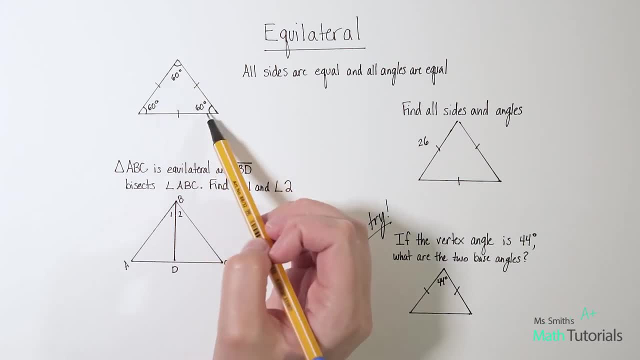 could be anything right, but we know the insides are 60 degrees. Alright, so let's do some examples. The first one says: find all sides and angles. Okay, so if I know, this is an equilateral triangle, as it shows me with the three tick marks right, and this side, it's telling me, is 26.. So I can.